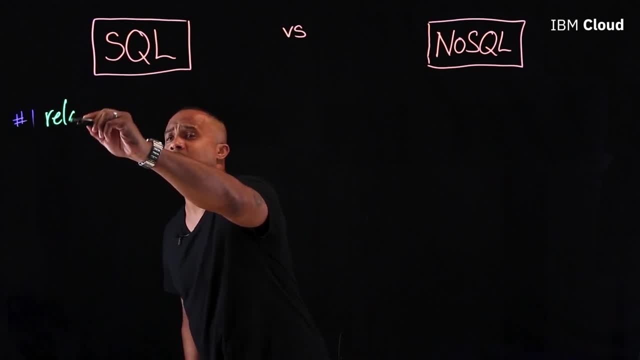 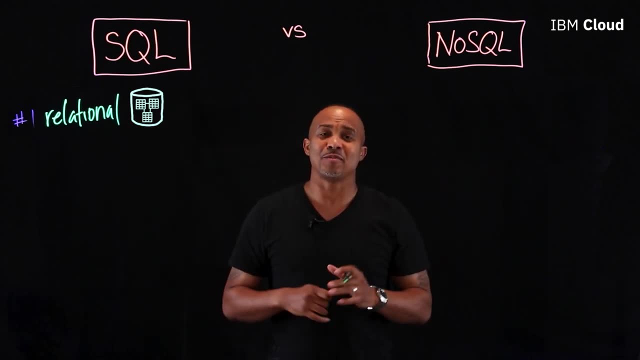 works off a relational database structure. here Now that means that you're going to access all your data points. They have to have some type of relation. You've got to do a lot of pre-work to kind of decide out your structure, how they're going to relate, Whereas on the NoSQL 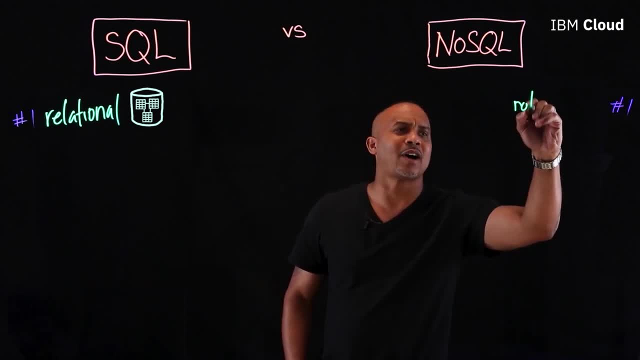 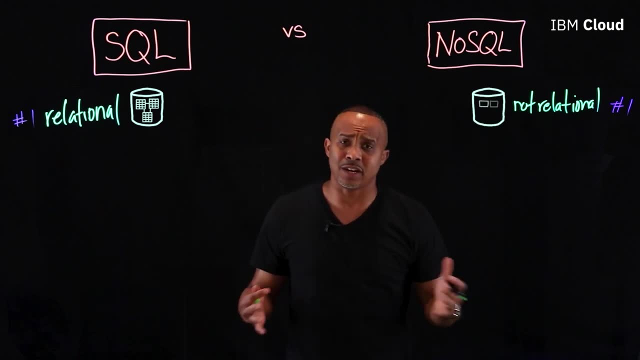 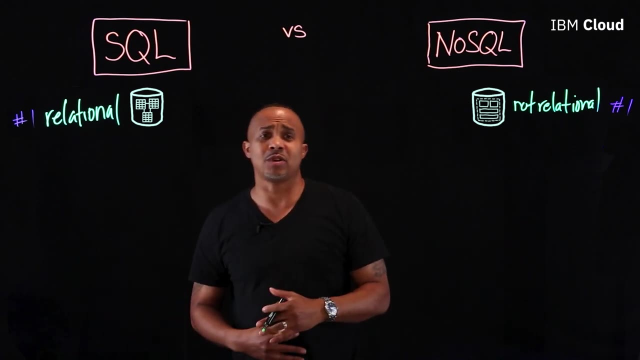 side. this is not relational so we really don't have to. I really feel for a lot of projects I can go ahead and get started and deal with a lot of that effort later on in the process here As your database kind of checks gets a lot of traffic and needs to really start to grow. 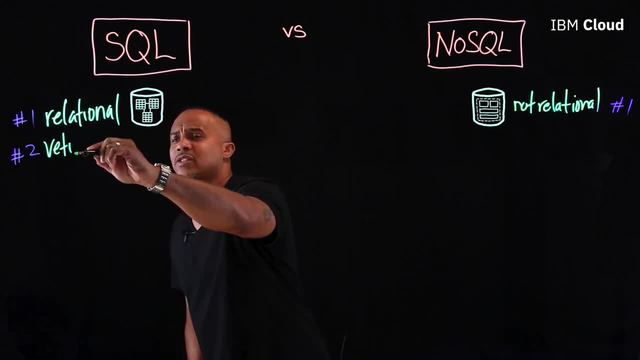 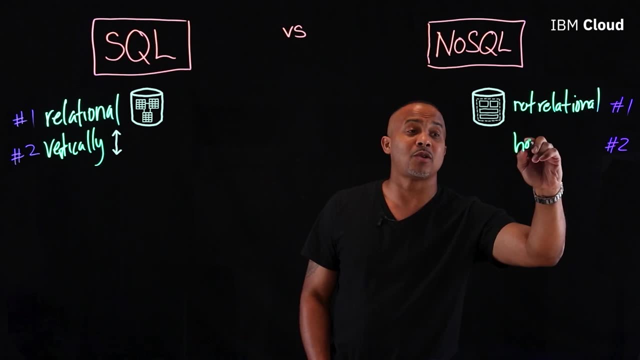 on the infrastructure for SQL servers, they're going to vertically scale, Okay- Whereas on the NoSQL side these are going to be horizontal. So I'm going to go ahead and get started, And I'm going to go ahead and get started. 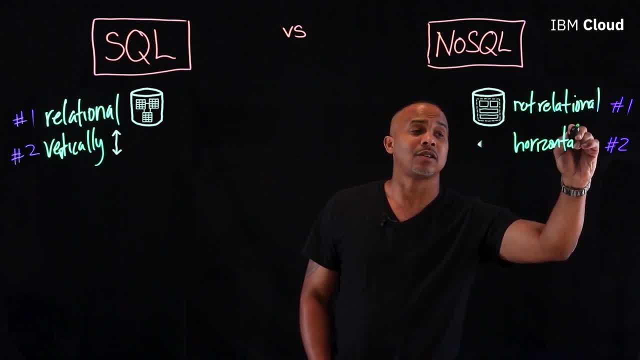 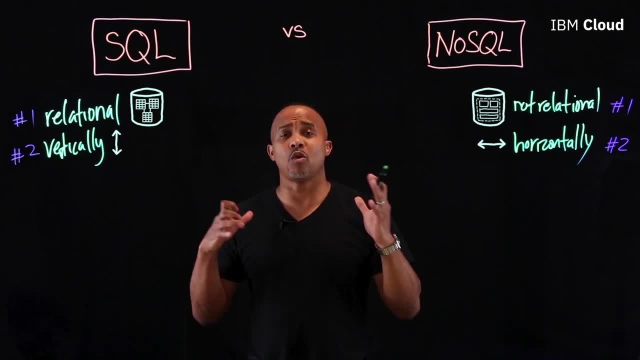 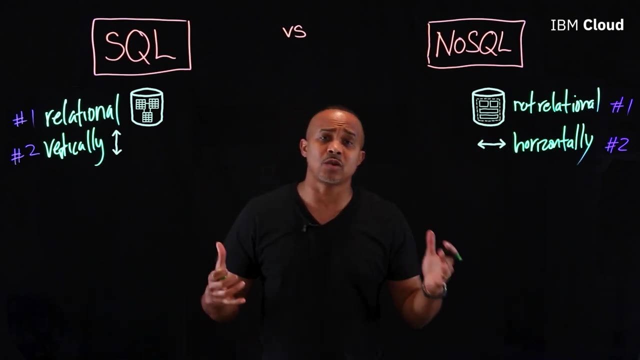 Horizontal Scaling, All right, And we know that SQL servers are going to be backed by disk. They're going to need more memory, more computing power to actually process all these transactions, Whereas horizontally, with NoSQL, it's all in memory. I can keep adding secondary. 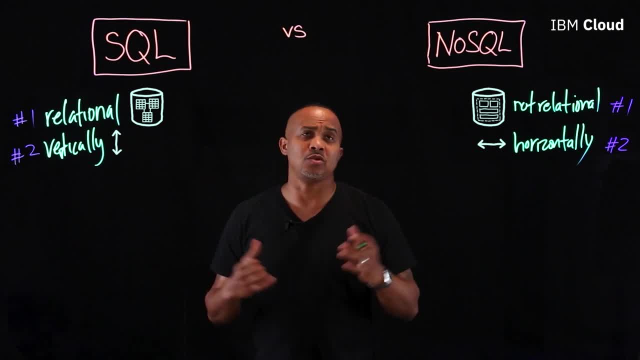 nodes to handle and balance out a lot of the usage there as well. On the SQL side, when I kind of talk about my structure, I'm going to go ahead and get started And I'm going to go ahead and get started. So I'm going to go ahead and get started And I'm going to go ahead and get started. 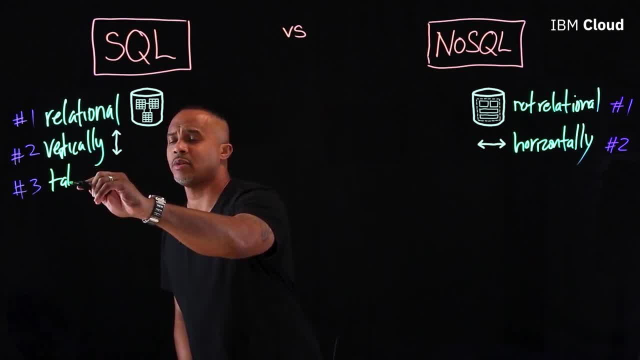 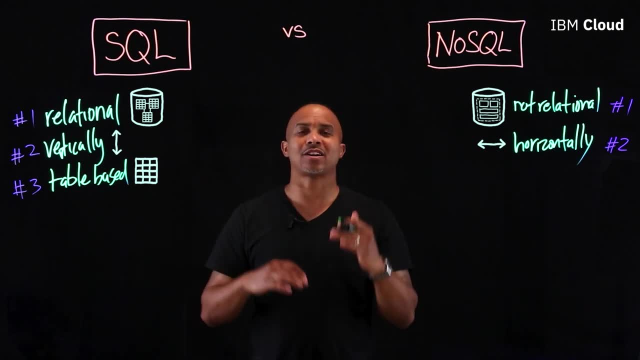 So I'm going to go ahead and get started, And I'm going to go ahead and get started. It's really going to be always about being table-based. I am super concerned about how I'm categorizing my entities, my tables, into records and how I'm doing. 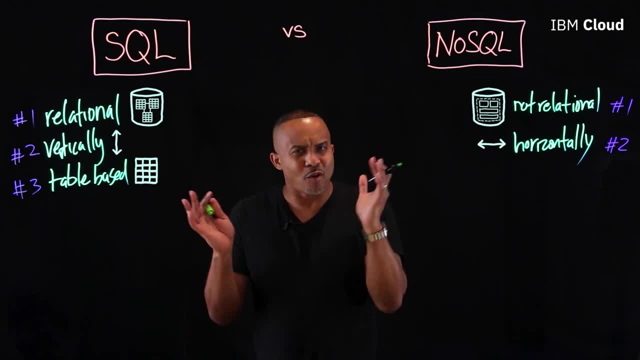 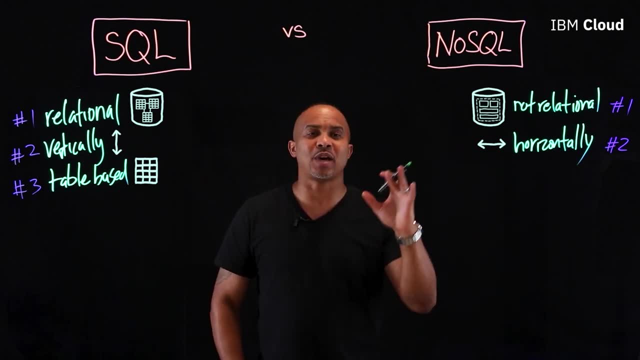 my relationships. So I have to kind of think of a- I like to say more of a warehouse kind of nature that I'm collecting all this data here as well. And we all know from NoSQL it is based on a document approach. So these are really going to be documents that are going to be used to 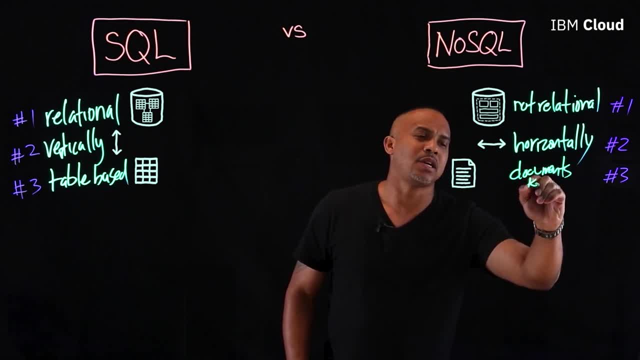 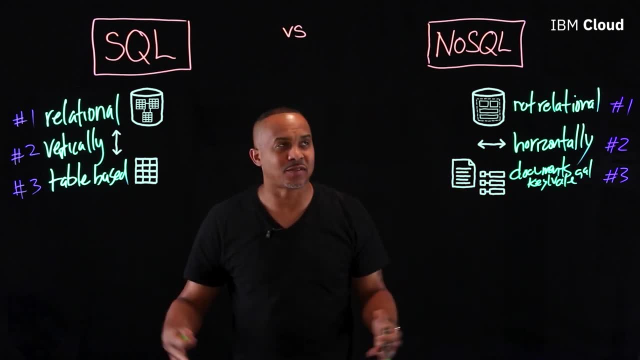 document. All right, they can be key value hashes. This is great for GraphQL. I mean a lot of the graphs. okay, it's really meant to not really have any kind of structure. It's kind of the opposite of being a table-based. I can fit pretty much anything in there as well, So what? 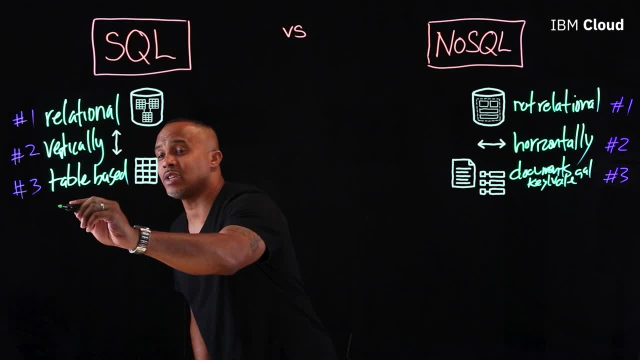 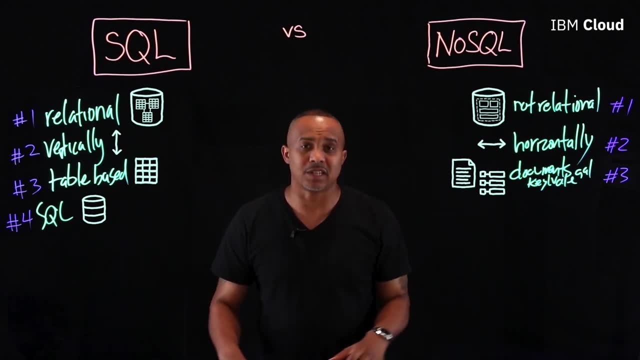 about when you want to access all the data. I'm going to have to use the SQL query language to actually define all my queries. I'm going to pull all my data out. So it's kind of some pre-planning about how I'm going to access and. 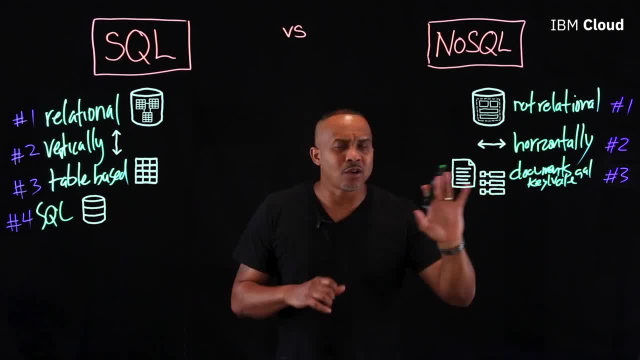 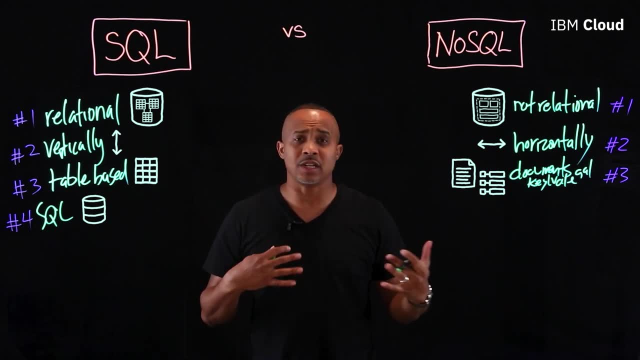 join my data. if I'm going to normalize all the data there, where I feel the NoSQL is definitely much, much more dynamic, All right, I'm really able to really just make my collections of these type of documents, no matter what the structure, and then I can have more freedom to let it flow and how I 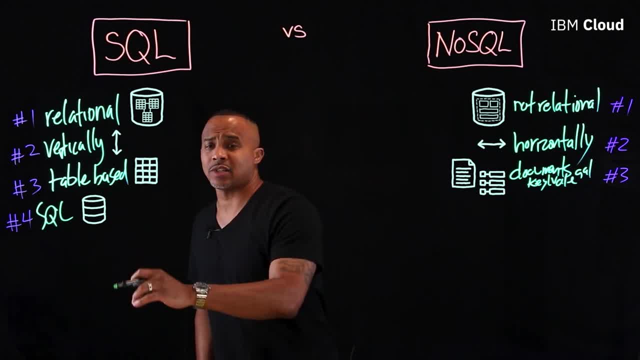 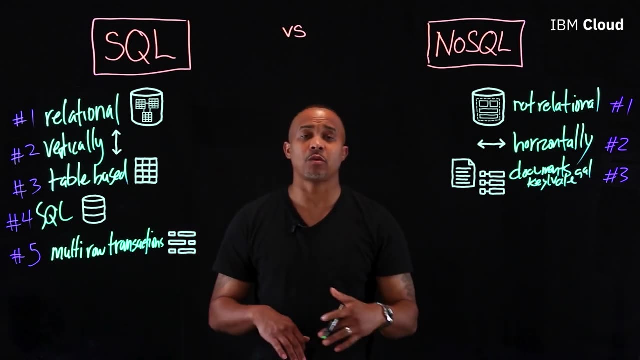 want to query these items as well. So, lastly, SQL: great for my data collection. Multi-row transactions where we have our tables. we have a lot of data that we want to put in. Remember the ability to do the transactions and being able to roll back and forth, So I can really 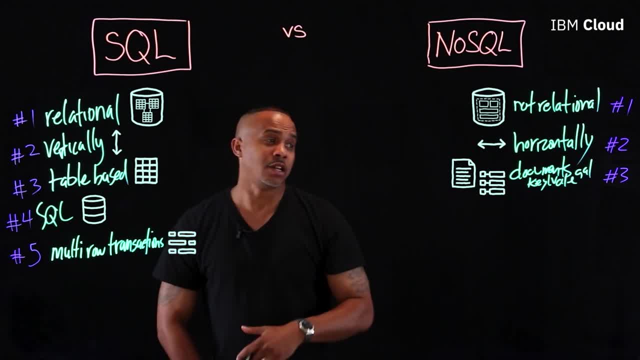 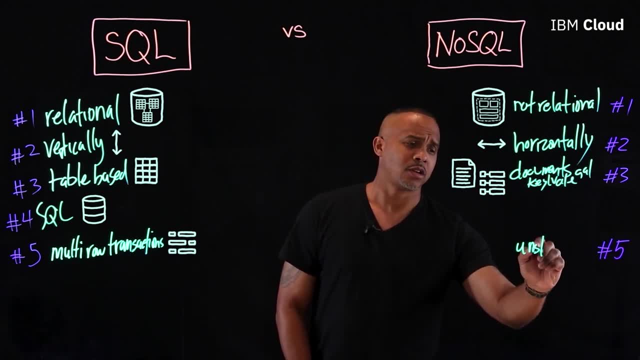 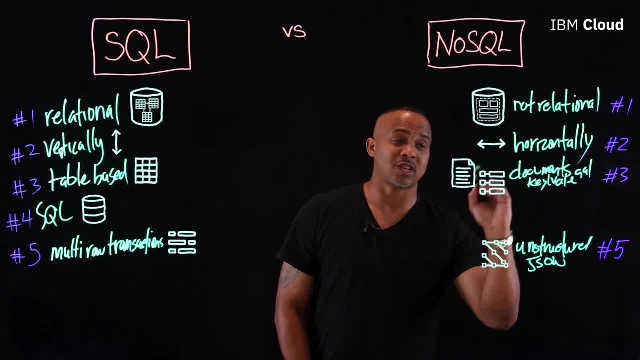 Okay, so I'm going to go ahead and do that. Okay, so I'm going to go ahead and do that. Usually it's JSON. It's very great for working with JSON. Let me make sure I write here in number four. 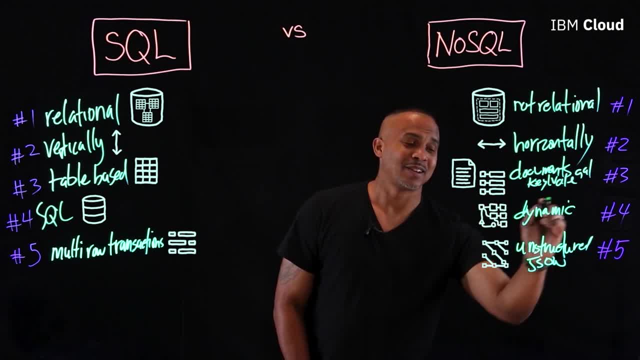 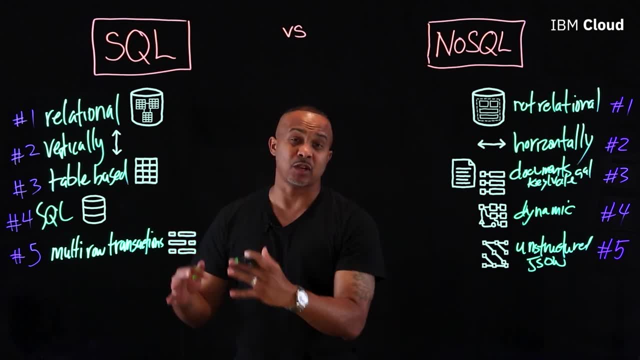 That was also dynamic. All right, so the unstructured JSON versus something that is very planned out. I specifically want to enter this in as well. So that kind of ends the features between the two, but actually I can think of a scenario where this: 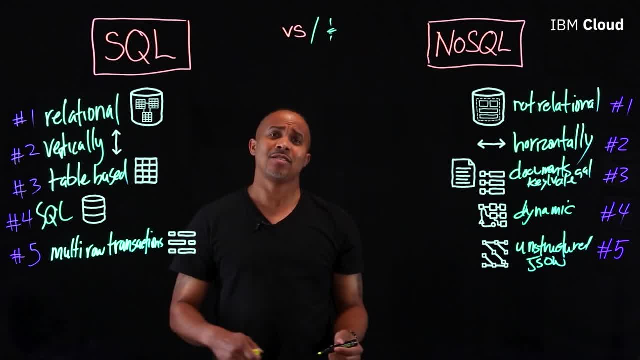 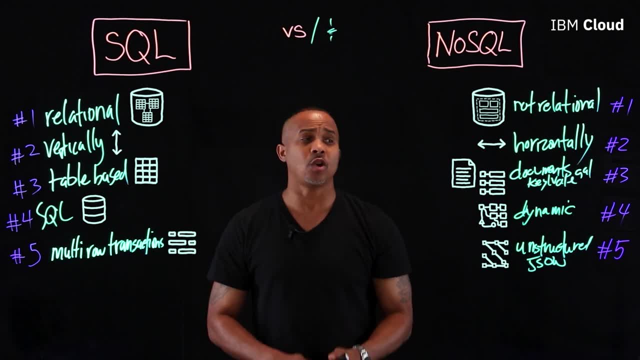 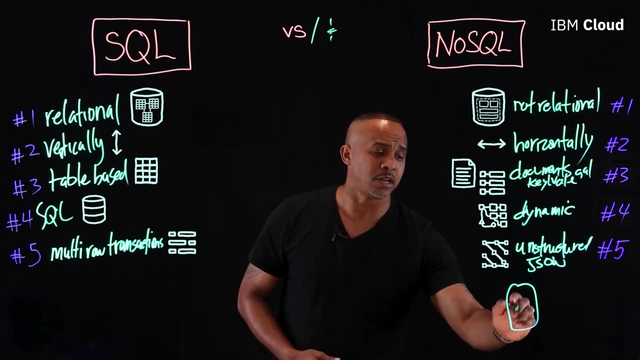 actually is an example, And that should be here as well. Do we really have to make a definitive choice of either or? One of those scenarios goes to the fact that I can have, let's say, I have- a common e-commerce application, which is usually composed of some bit of mobile. 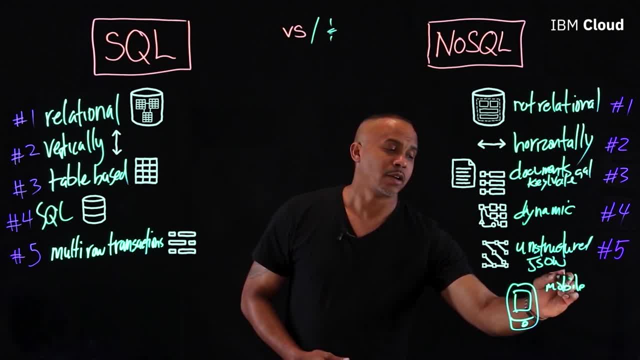 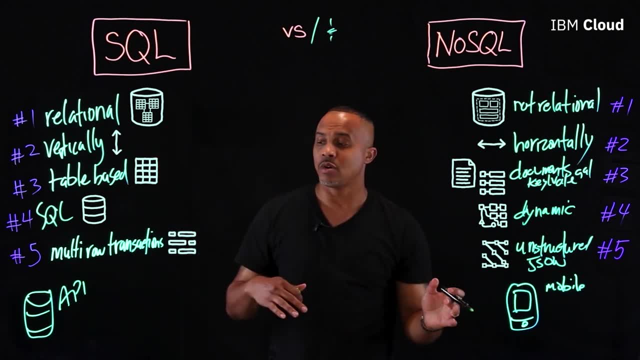 and has some interaction with more of a back-end, whether it's an API that wants to kind of go: we want to commit a lot of the data. Think about a shopping cart. Okay, let's kind of visualize this for a minute.